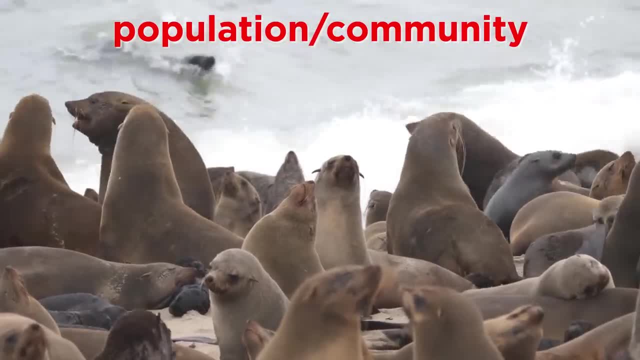 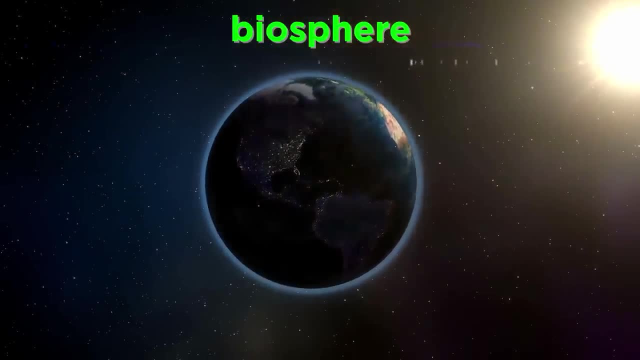 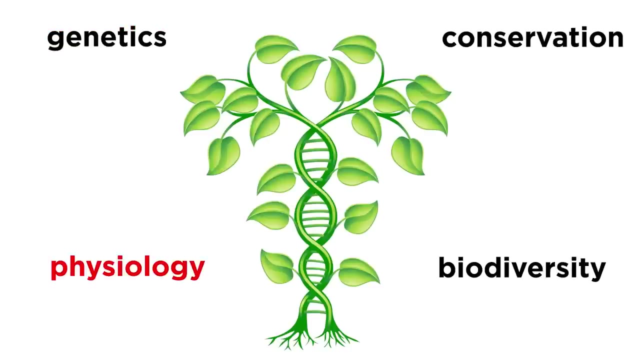 organism itself, populations or communities of organisms, large ecosystems or even the entire biosphere as a whole, which is a word that refers to the regions of the planet occupied by living organisms. They can specialize even further, focusing on genetics, plant and animal physiology. 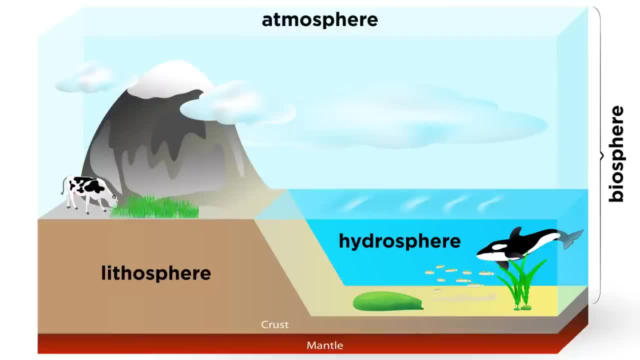 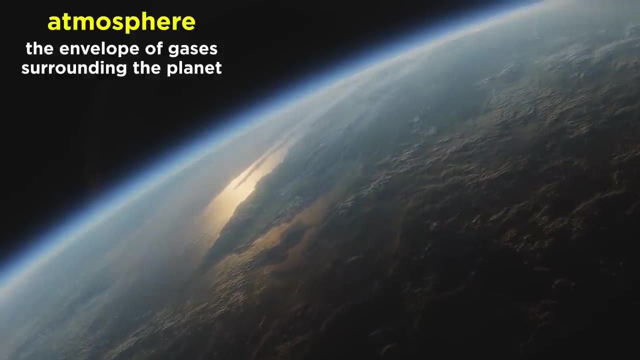 biodiversity or conservation. As we are beginning to understand, the Earth can be broken down into distinct spheres, such as the atmosphere, lithosphere, cryosphere and biosphere. We define the atmosphere as an envelope of gases surrounding the planet making it habitable for life. The lithosphere is the rigid outer part of the Earth, consisting 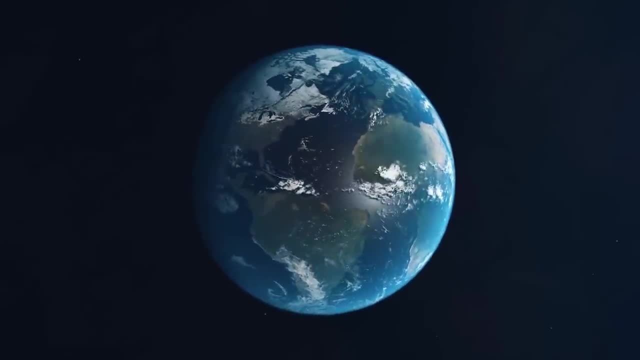 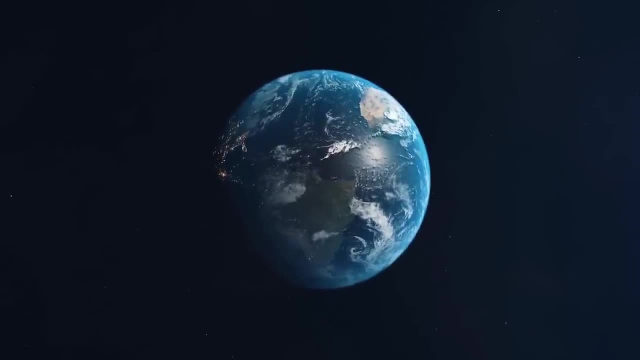 of the crust and upper mantle Over geologic timescales. the lithosphere determines how much land is available for living organisms to inhabit and where that land is located geographically. The, The cryosphere, is the part of Earth's surface characterized by frozen water. 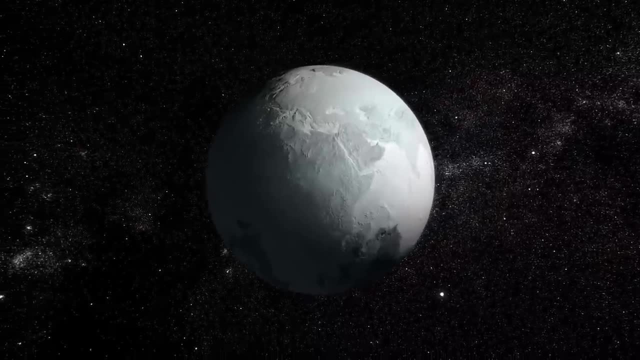 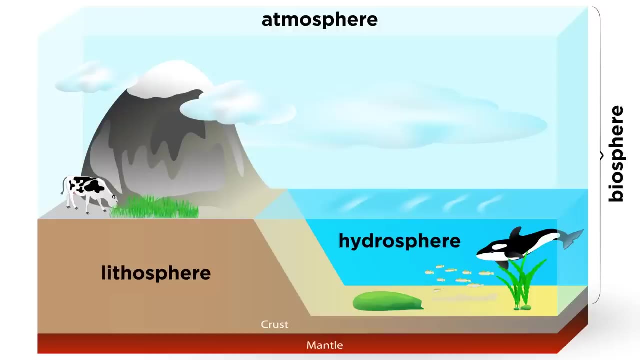 Its expanse changes over time, and this is an important factor in maintaining a habitable climate. And then the biosphere we described a moment ago. These spheres are dynamic and can influence one another, so the better we understand interactions within individual spheres, the more equipped we are to understand how they all work together. 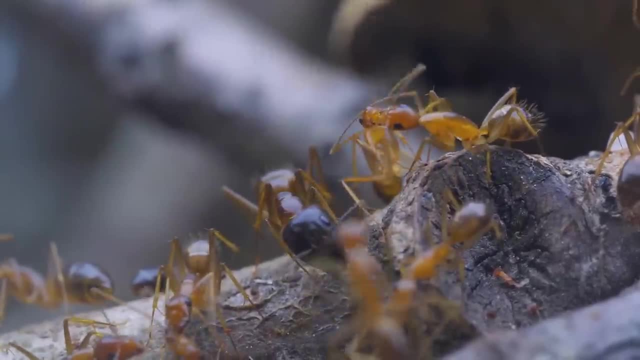 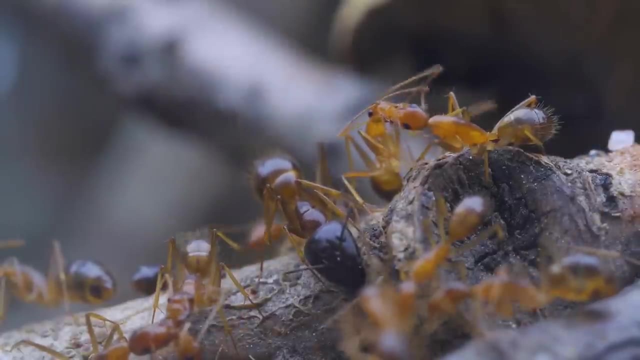 as an entire system. But let's zoom back in for a moment. In any given physical environment, ecologists seek to study both the types of organisms present and their abundance. By monitoring these factors over time, ecologists can track the general trends and well-being. 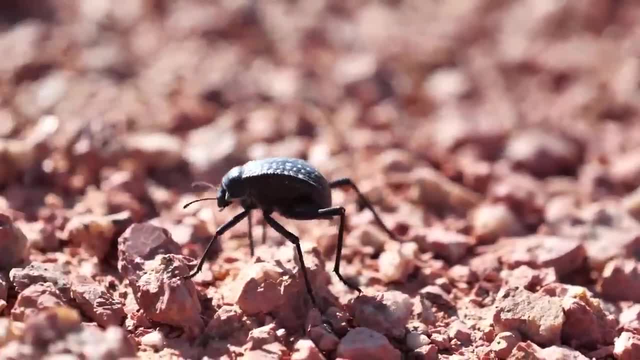 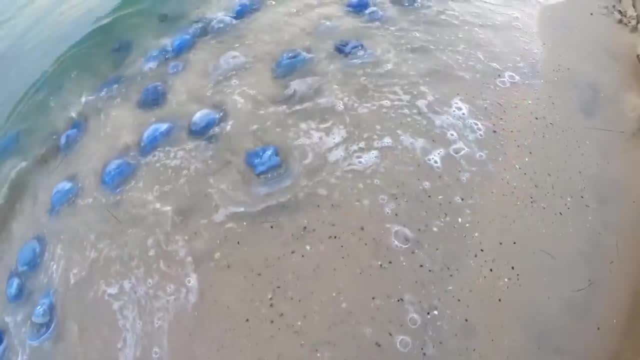 of the ecosystem. For example, as climate changes, the numbers and types of organisms may change too in order to adapt to changing conditions. This might result in a positive or negative change, depending on the species, and as a whole, the ecosystem could be accordingly fortified and the environment could be more. 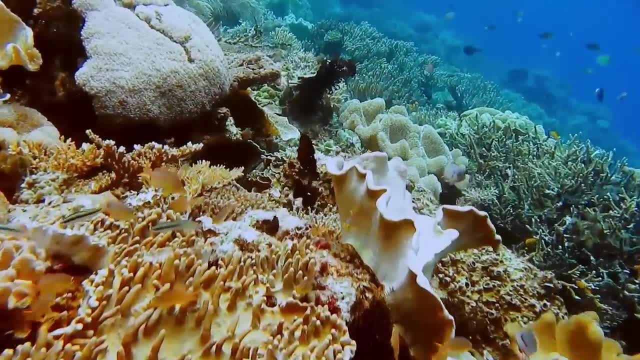 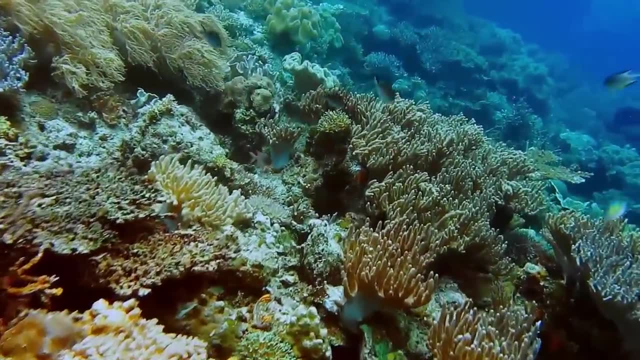 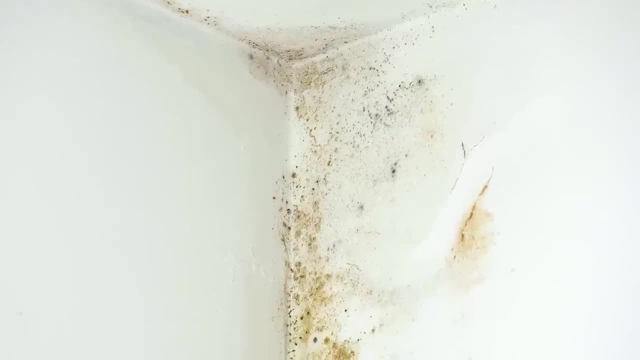 polluted or placed in jeopardy. The more we know and understand about interactions between organisms and their environments, the better we will be able to address any consequences that arise. Ecology does not encompass only the outdoors, as many might assume. What about mold in your kitchen or shower? 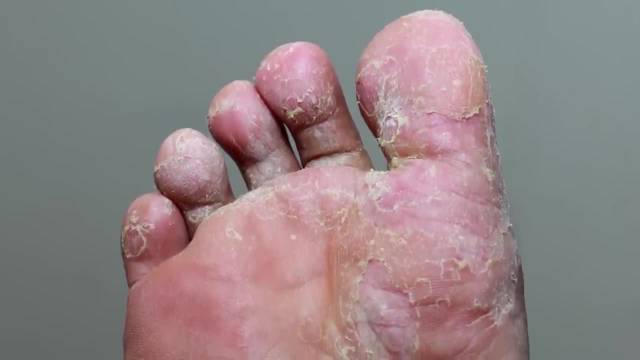 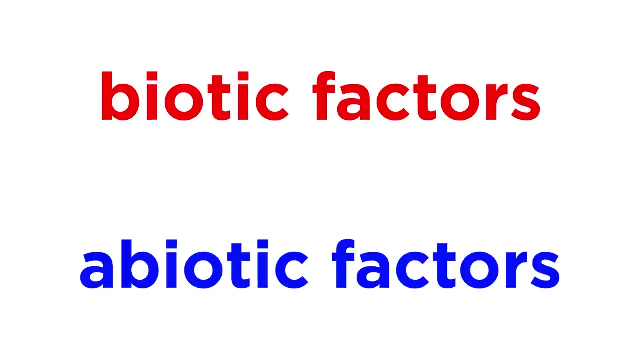 Or if you're an athlete, the dreaded athlete's foot fungus that you can pick up in a locker room. These are also examples of ecology in action. factors that can affect the distribution of organisms can be biotic or biological, So let's take a look. 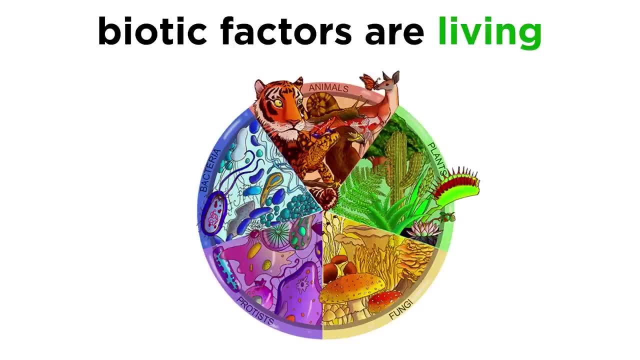 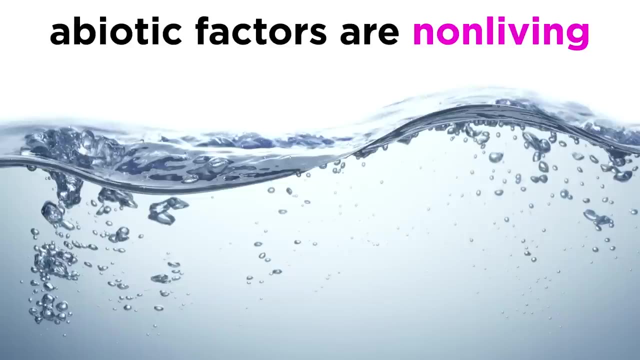 Biotic refers to the living factors, which can include animals, plants, bacteria and fungi, like the athlete's foot fungus. The fungus is living, but how did it grow in the first place? Water Availability of water is abiotic or a non-living factor. 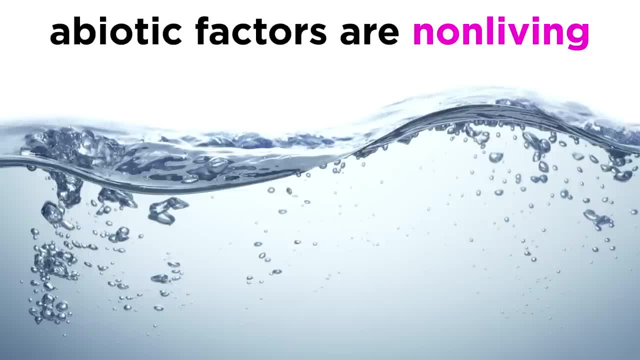 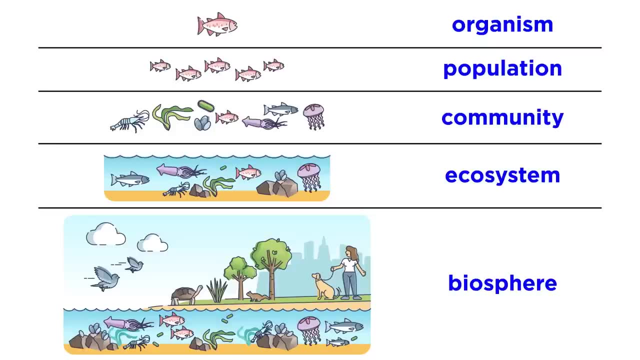 These are physical or chemical in nature and they also impact an ecosystem. A few other examples include air, soil and sunlight. Earlier we mentioned the rain, the wind and the sun. We also mentioned the range in scale of phenomena that ecologists can study. 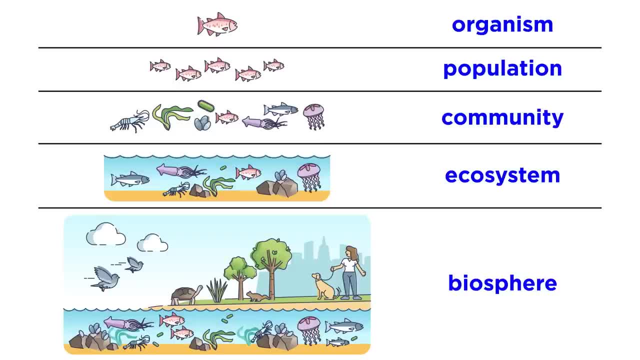 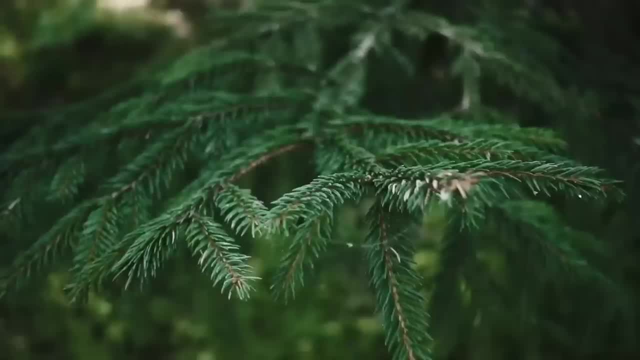 Later we will examine this more thoroughly, but let's briefly summarize the tiers now so that you know what to expect moving forward. Think of an individual tree, Let's say a pine tree. For those ecologists who are detail-oriented and like studying the small scale they might. 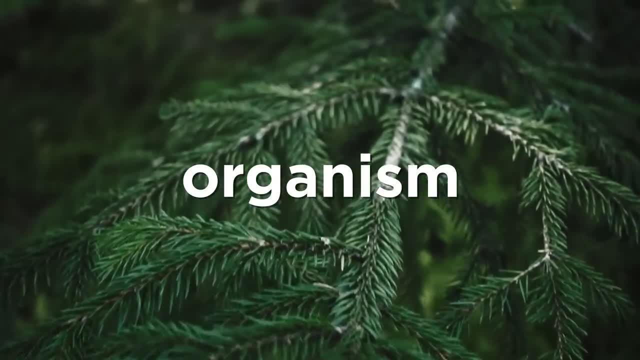 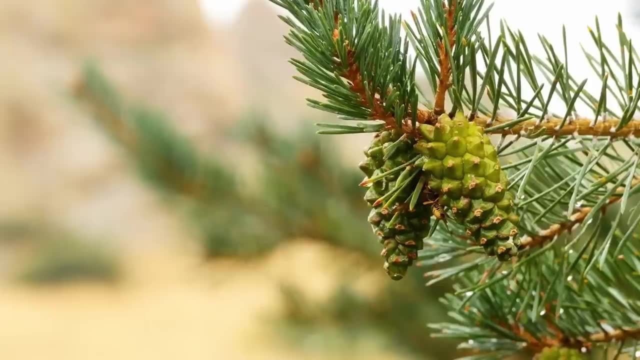 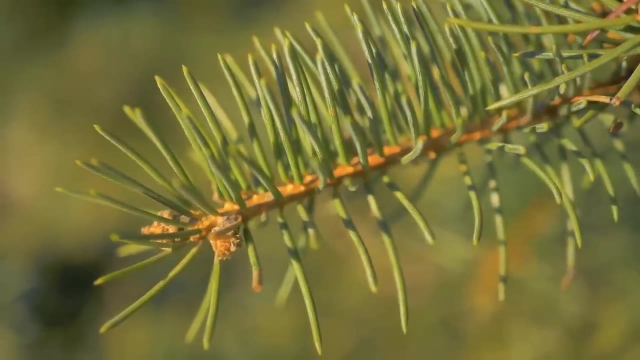 be more inclined to study ecology at the organism level. They're interested in details like how this pine tree adapts and how natural selection played a role in the evolution of beneficial features for survival. Organism ecologists study not only the physiological traits of an organism or those traits that 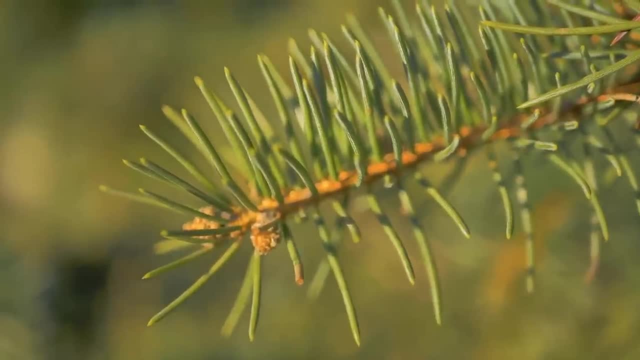 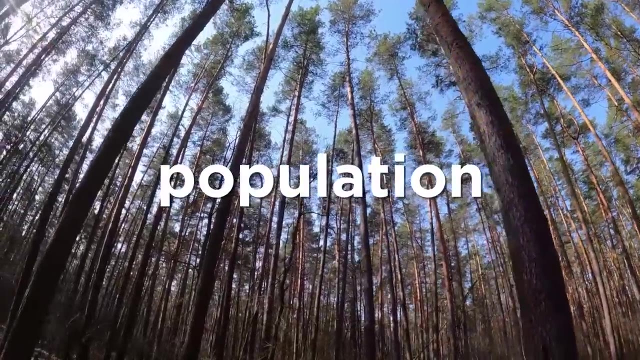 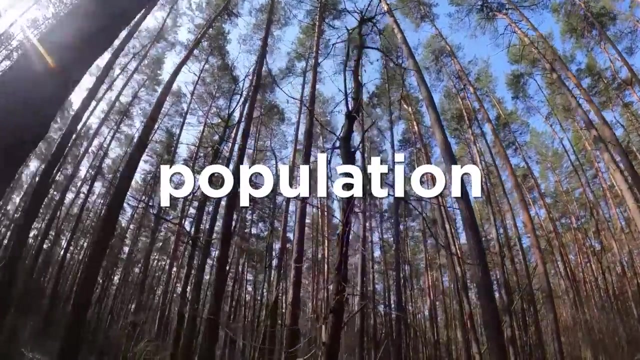 relate to normal functions of living organisms and their parts, but can also focus on organism behaviors. Next on our scale is populations or groups of organisms of the same species that live in the same area at the same time. So all of the pine trees living in a specific area make up a population. 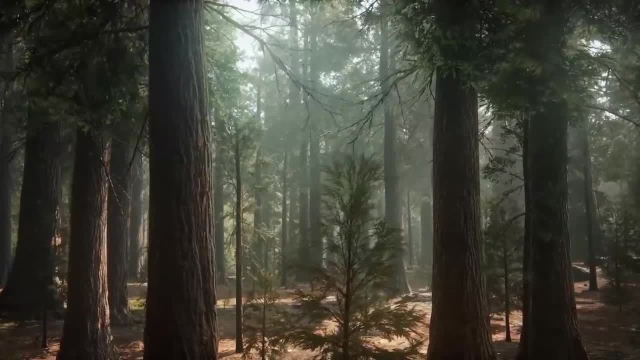 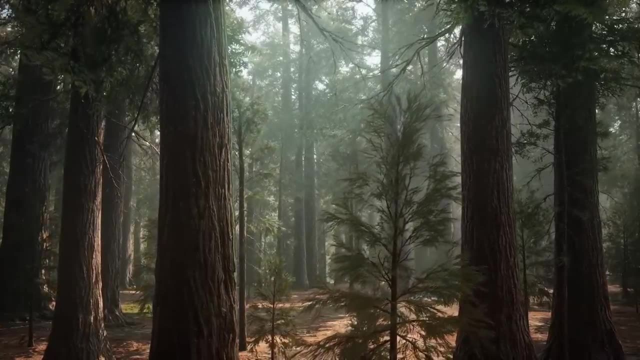 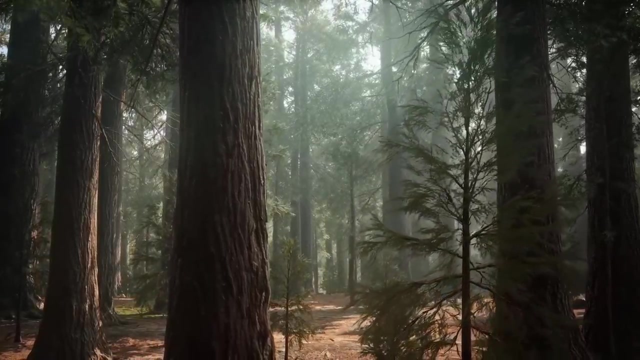 Population. ecologists are interested not only in the size of the population or the number of pine trees, but also the densities and structures of these populations and how they change with time. How many trees are adults? How many are juveniles or seedlings? 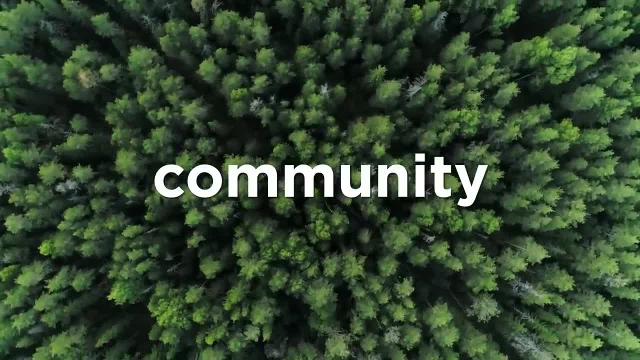 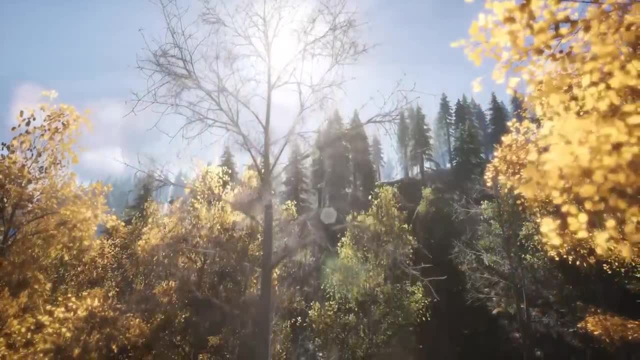 Next comes communities. What do we mean by this term? in the ecological sense, A biological community is defined as all the populations of different species that live in a given area. So now we're looking beyond the pine trees. What other tree species are there? 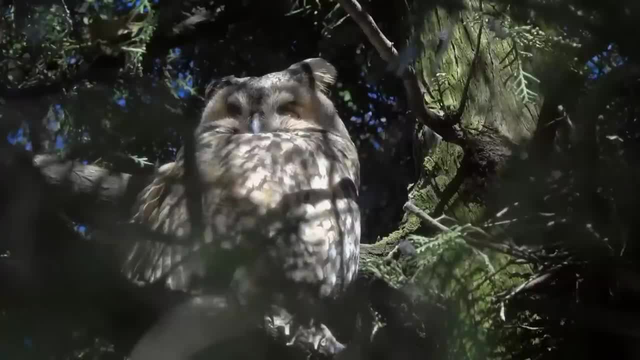 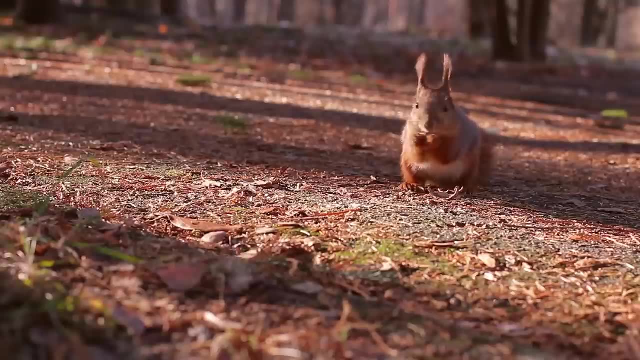 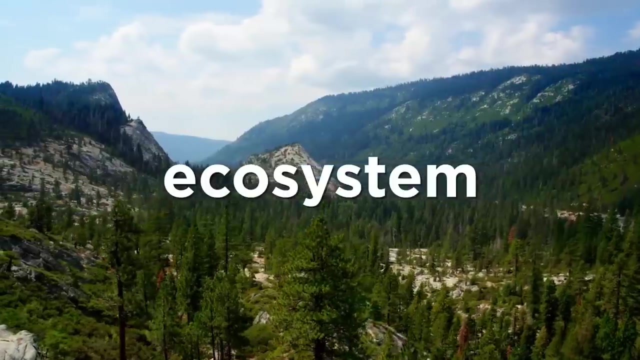 And what other organisms call this area home? Which other plants, Which animals, Which bacteria? Community ecologists are interested in studying the interactions between populations of species, and then how those interactions shape the entire community. Let's zoom out again. What about an ecosystem?